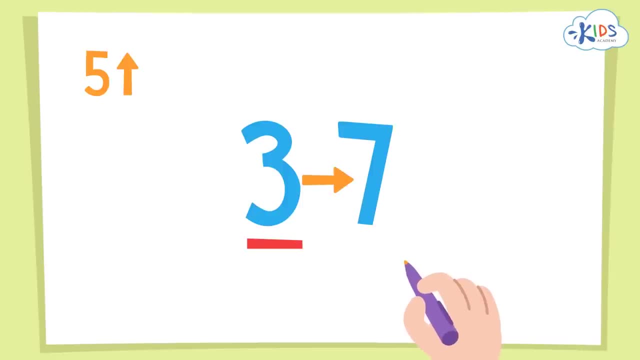 in the 1s place. Since that number is a 7, we're going to round up because 7 is greater than 5.. We'll round 37 up to 40.. You round the number in the 10s place and make the number in the 1s place a 0. 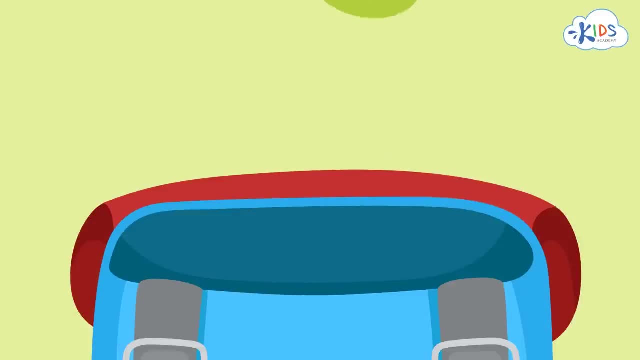 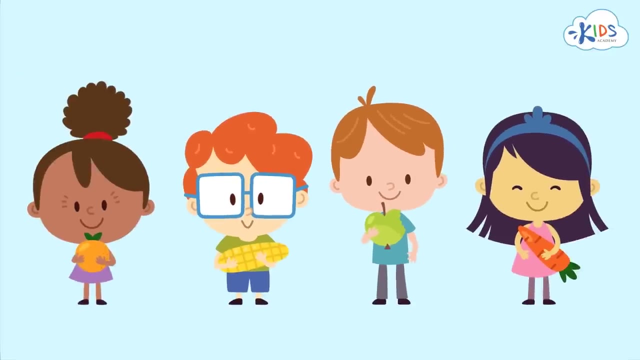 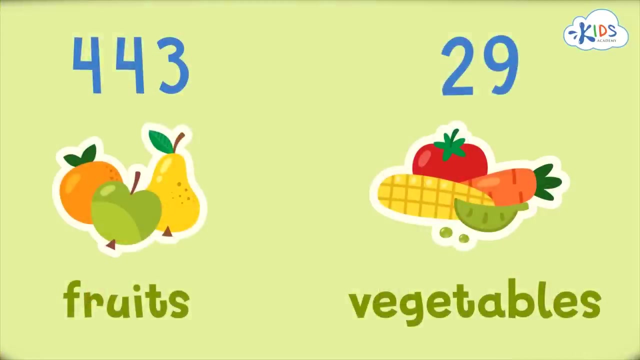 Let's take a look at a real life situation that requires rounding and see how our rounding to the nearest 10 and 100 skills can come in handy. These kids want to see how many fruits and vegetables their class has eaten this week. Let's help the kids figure this out quicker by rounding. 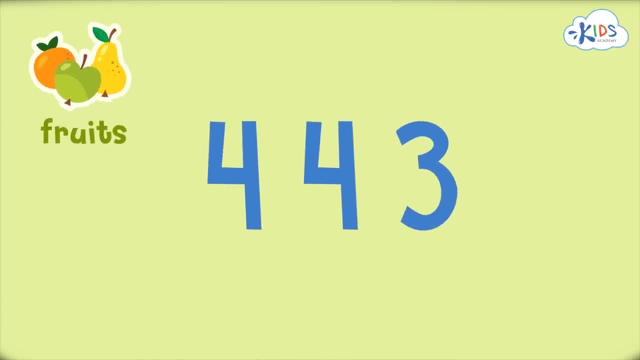 First, we'll round the fruits eaten this week. According to the data, 443 pieces of fruit were eaten this week. Now let's round this number to the nearest 100.. We'll use the strategy of underlining the 100s place and drawing. 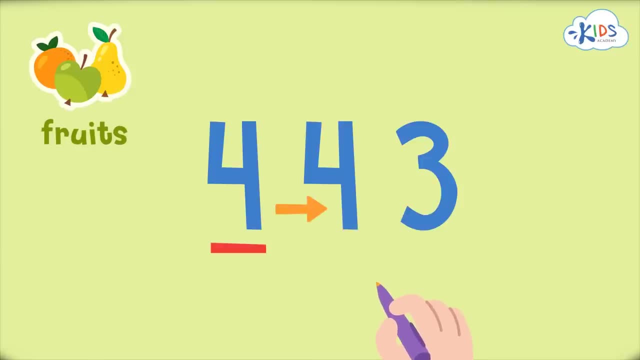 an arrow to the 10s place so we know what numbers we have to look at. I see a 4 in the 10s place. I know if it's 4 or lower. we have to round down. The 4 in the 100s place is underlined, So we have to round the 4 in the 10s place. We'll 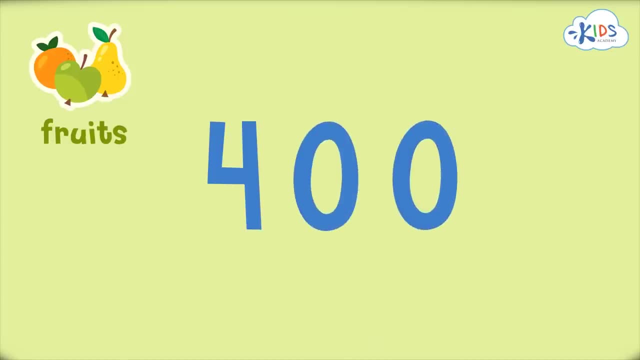 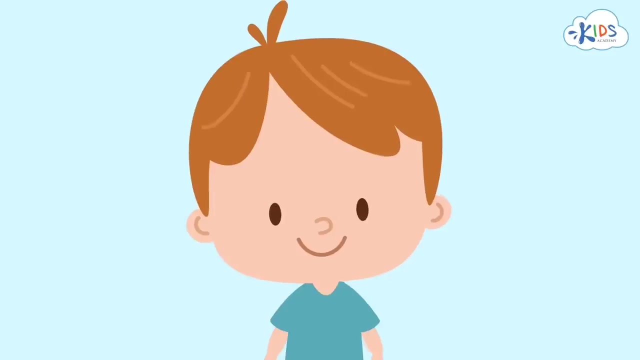 round the 4 in the 100s place to 400.. When rounding to the 100s place, the number in the 10s and 1s place become 0s. Now I know about 400 pieces of fruit were eaten this week. 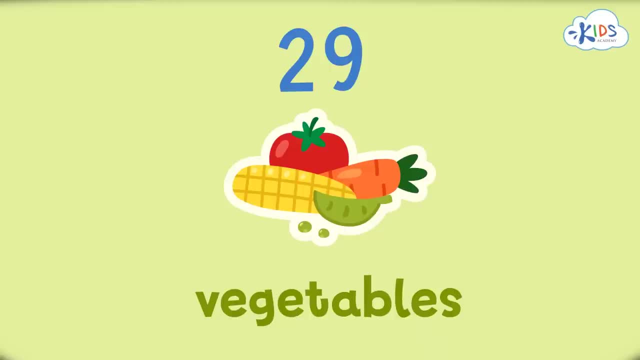 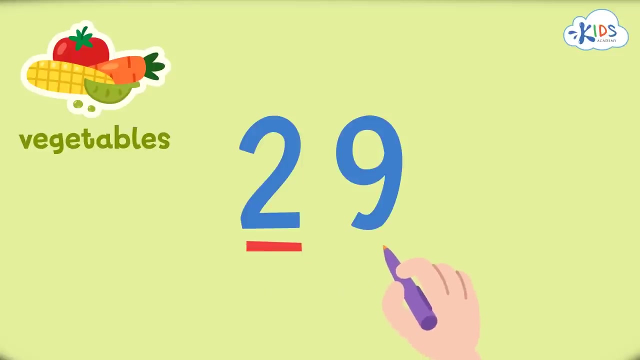 Next, we'll round the vegetables eaten this week. According to the data, 29 vegetables were eaten this week by kids Man. these kids need to eat more veggies. Now let's round this number to the nearest 10.. We'll use the strategy of underlining the 10s place and drawing an arrow to the 1s place. 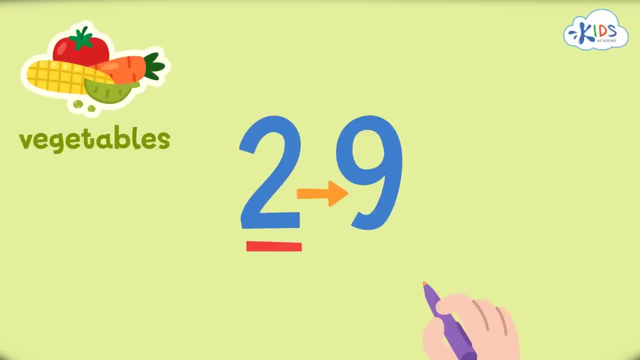 so we know what numbers we have to look at. I see a 9 in the 1s place. I know if it's 5 or higher. we have to round up. The 2 in the 10s place is underlined, So we have to round the 2 in the 10s to 3 10s. 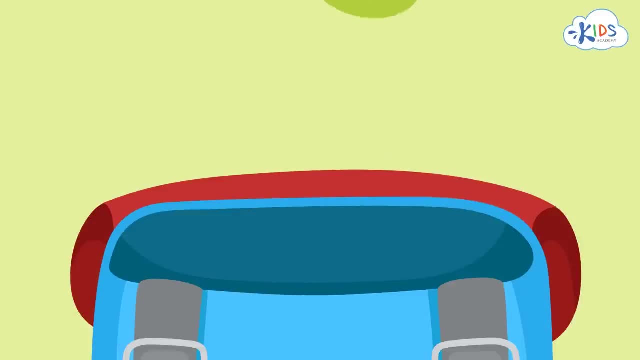 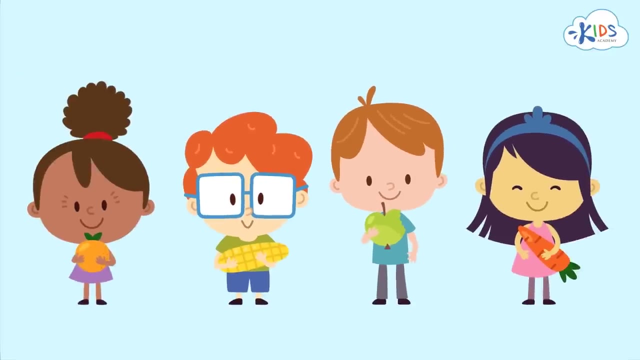 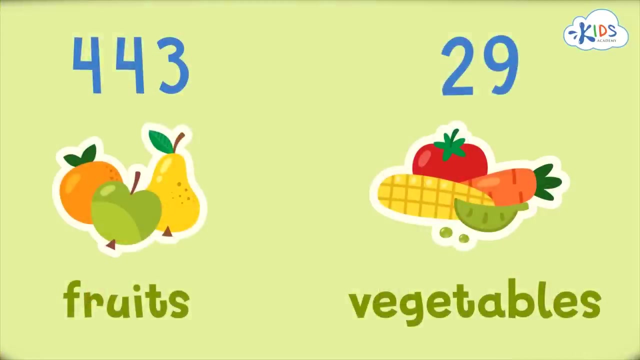 Let's take a look at a real life situation that requires rounding and see how our rounding to the nearest 10 and 100 skills can come in handy. These kids want to see how many fruits and vegetables their class has eaten this week. Let's help the kids figure this out quicker by rounding. 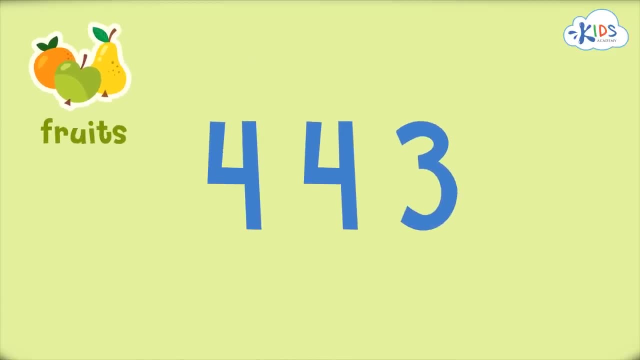 First, we'll round the fruits eaten this week. According to the data, 443 pieces of fruit were eaten this week. Now let's round this number to the nearest hundred. We'll use the strategy of underlining the 100s place and drawing an arrow to the 10s place, so we know what numbers we have to look at. 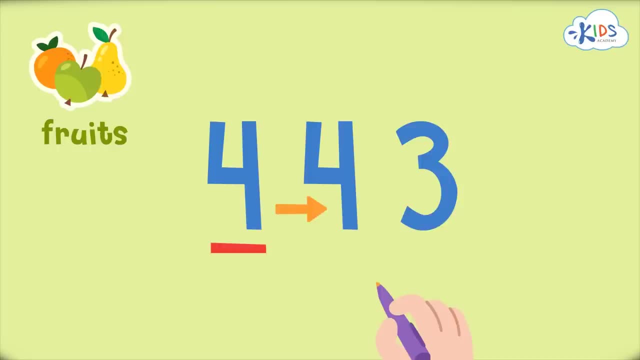 I see a 4 in the 10s place. I know if it's 4 or lower. we have to round down. The 4 in the 100s place is underlined, so we have to round the 4 in the 1s place. 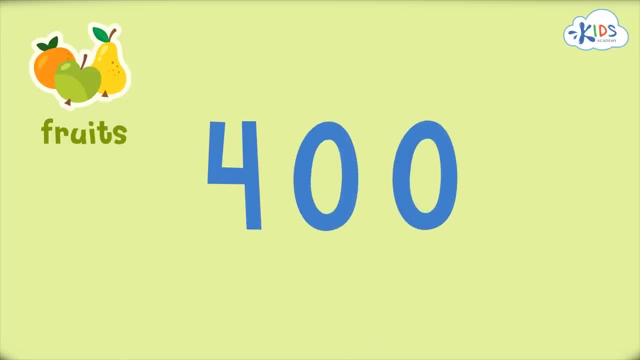 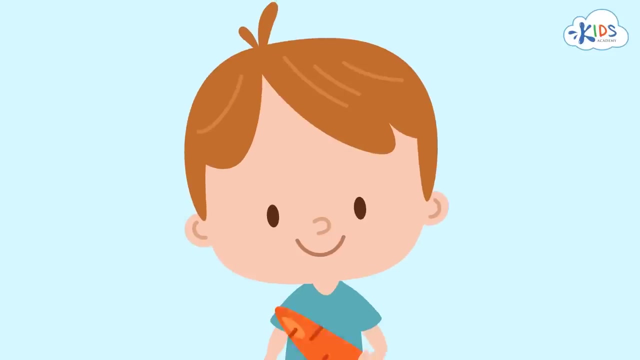 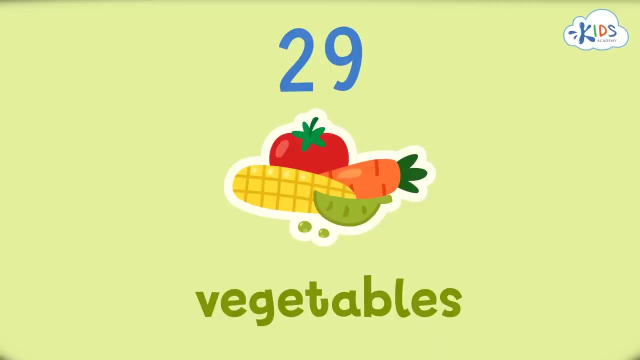 four in the hundreds place to four hundred. When rounding to the hundreds, place the number in the tens, and ones place become zeros. Now I know about 400 pieces of fruit were eaten this week. Next we'll round the vegetables eaten this week. According to the data, 29 vegetables were eaten. 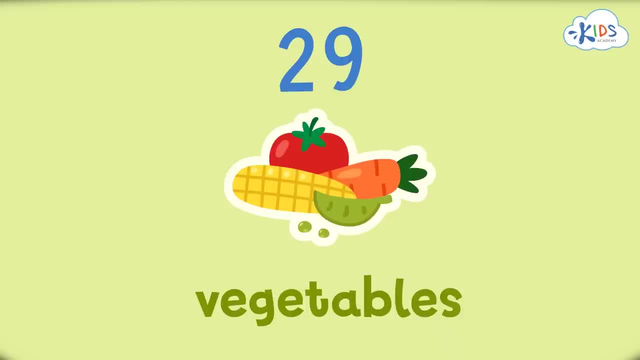 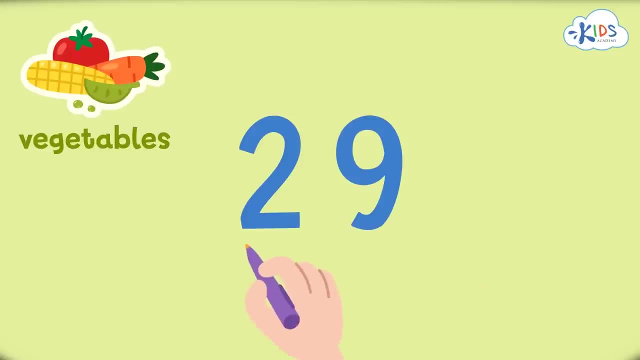 this week by kids Man. these kids need to eat more veggies. Now let's round this number to the nearest ten. We'll use the strategy of underlining the tens place and drawing an arrow to the ones place, so we know what numbers we have to look at. I see a nine in the ones place. I know if it's five. 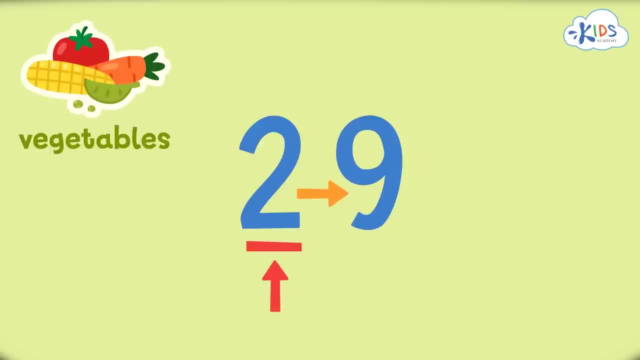 or higher. we have to round up. The two in the tens place is underlined. so we have to round the two in the tens to three tens. When rounding to the tens place, the number in the ones place becomes a zero. Now I know the kids. 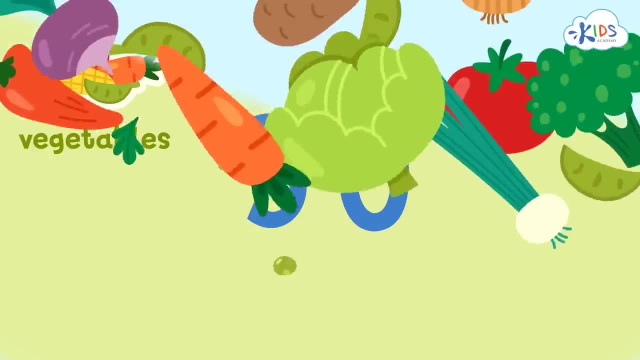 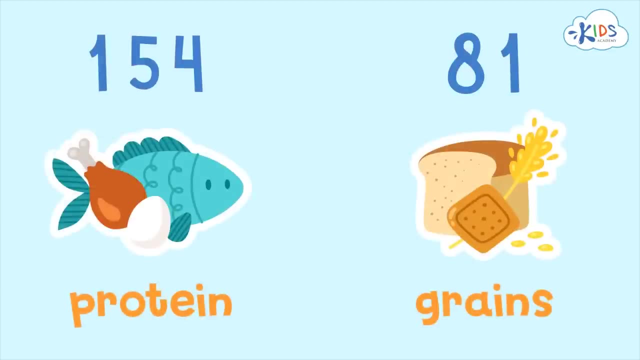 only ate about 30 vegetables this week. I'll leave you with a challenge. I want you to help the kids round the next two types of food one kid eats a day, to the nearest hundred and ten. I'll give you some time to think, but if you need more time you can pause the video and answer when you're ready.